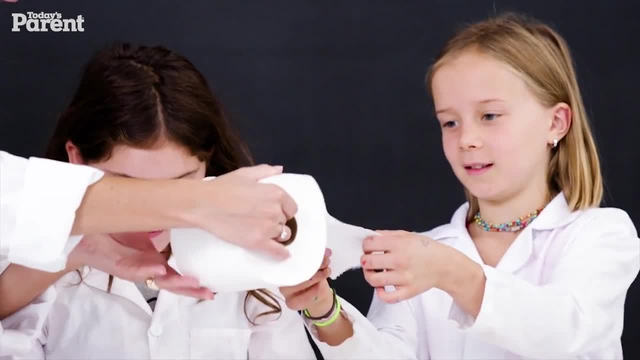 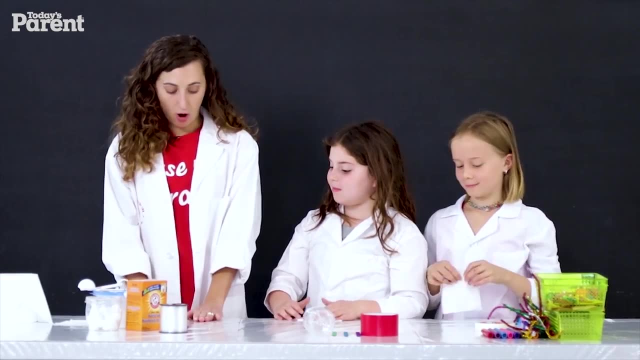 One, two, awesome. Okay, It's a perfect square, Ready. Great job, I can eat it. Okay. the next thing is put them down on the table like a placemat, And then I want you to get your measuring spoons, and we're going to use one teaspoon. 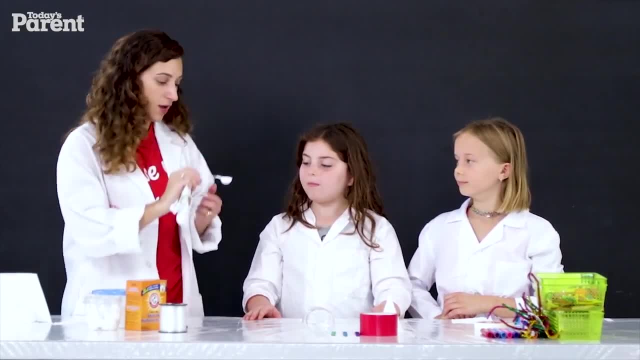 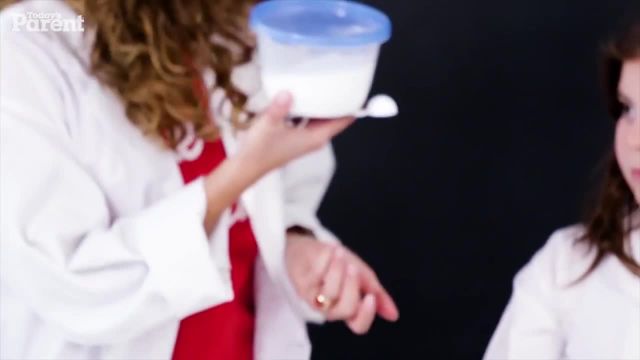 just like this, And I think you probably have these at home somewhere in the kitchen. So we're going to use baking soda Just like this. But I happen to have my baking soda already in a Tupperware, so we'll just scoop it out of here. Okay, Mila, you go first and then we'll pass it over to Sophie. 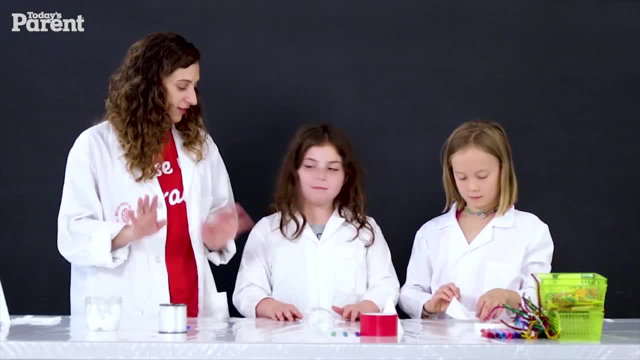 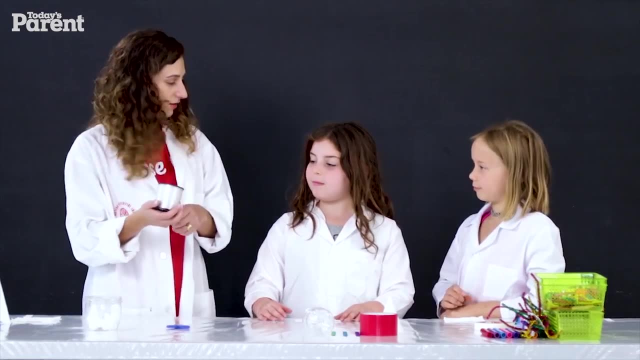 That's great. Does everyone have the baking soda right in the middle of their toilet paper, Kind of in the middle? Yeah, that looks good. Yeah, that looks great, Okay. so the next thing. this is a bit complicated and I'm here to help. 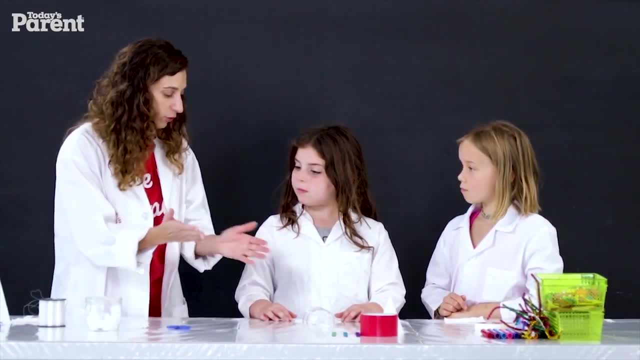 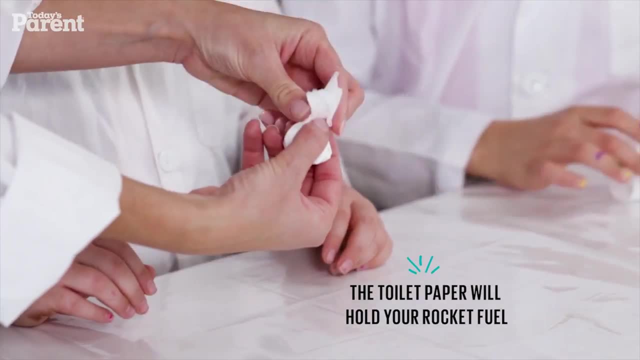 but we'll try it ourselves. What I want us to do is we're going to actually kind of fold it together, Almost create like a little bag. And then do you see here, Sophie, do you see how I have it crunched together like that? If you can hold it like that for me, 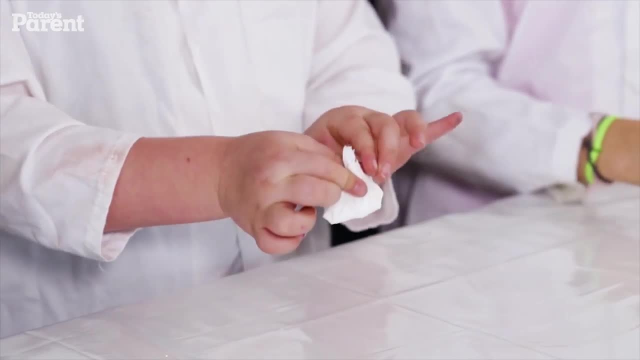 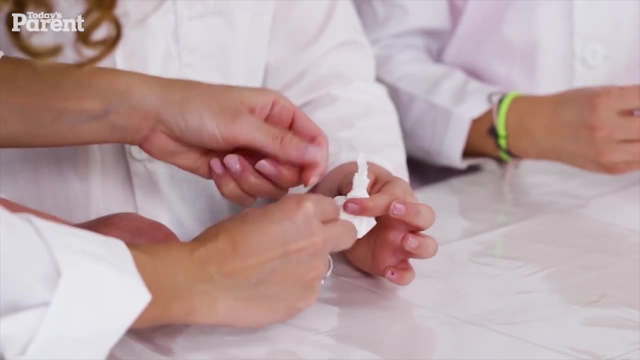 I'm going to get ready and I'm going to bring some string to tie it together. And then, Mila, will you hold it like that, Just like that. That's awesome, Okay, and I'm going to come around and use this string to tie it up. You keep your fingers there. 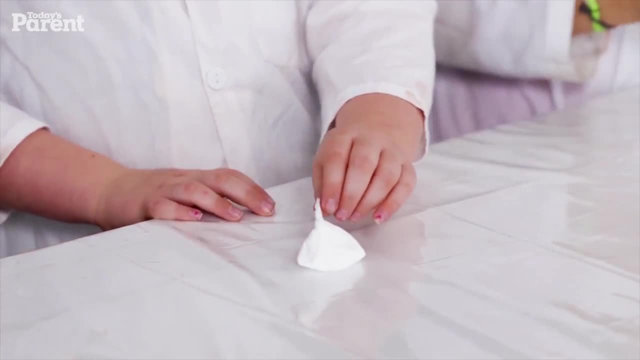 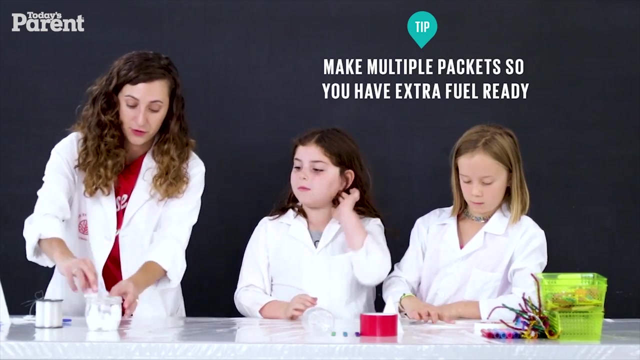 Okay, and I'm just going to cut off the extra ones because these are a bit long. Okay, Mila, can I get a high five? Yes, These are going to be really important to propel our rocket up into the air. I'm going to put them to the side for now. 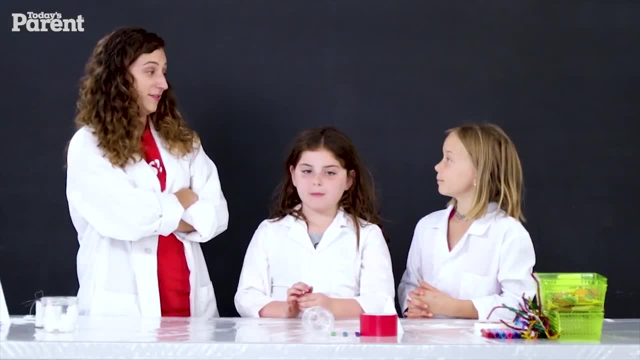 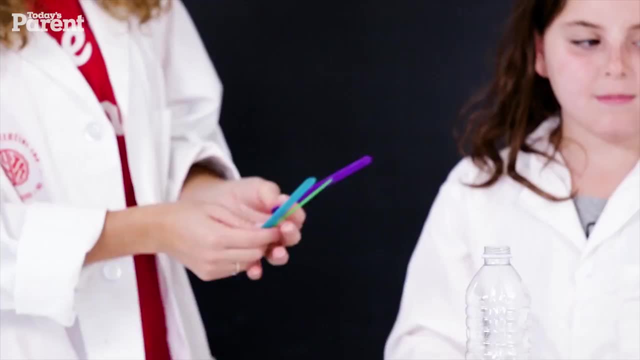 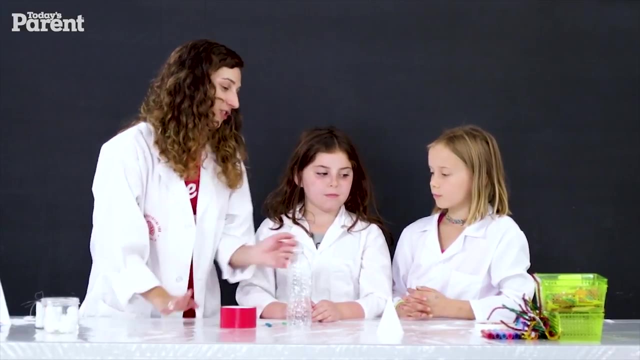 Do you know what the next step is? It's actually building, So we're going to use a water bottle, any old water bottle, and then you're going to have three Popsicle sticks and also awesome duct tape and also one other thing. This is just a little addition that I like to do. 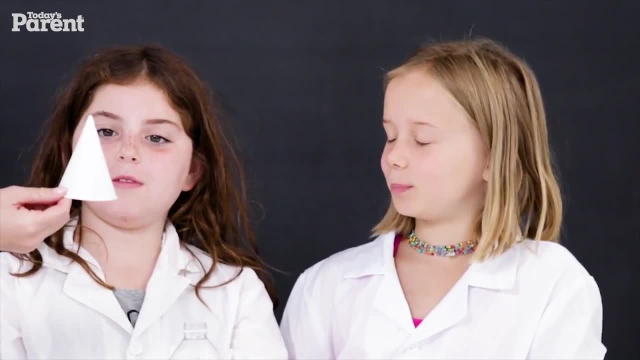 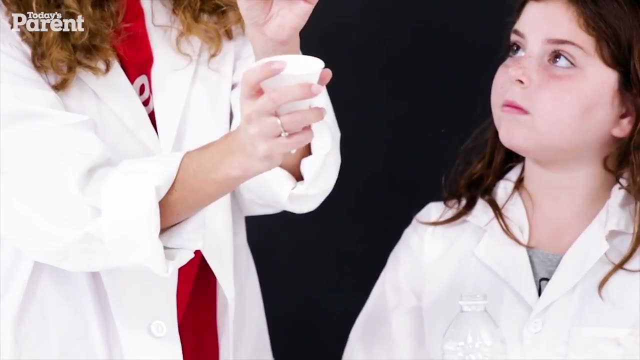 Does anyone know what this is? Popsicle sticks? It's a tap, It's a cup, It's a paper cup. Sometimes you get this and you see them in offices or at homes and you have, like you know, a water jug at home that you can pour your water in Well. 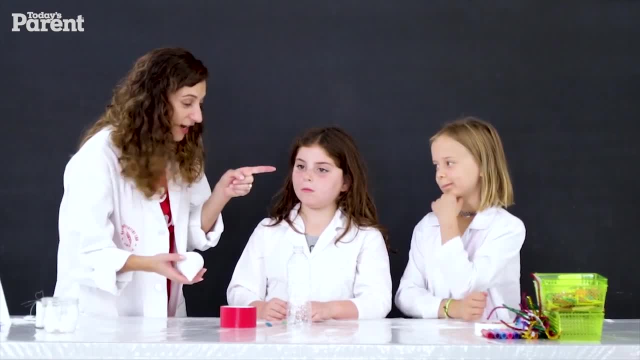 this, I thought: Is it a funnel? Well, not exactly as a funnel, but that's a great idea. I thought it would be fun if we use it as the very top of our rocket, so it helps it direct go up into the air. 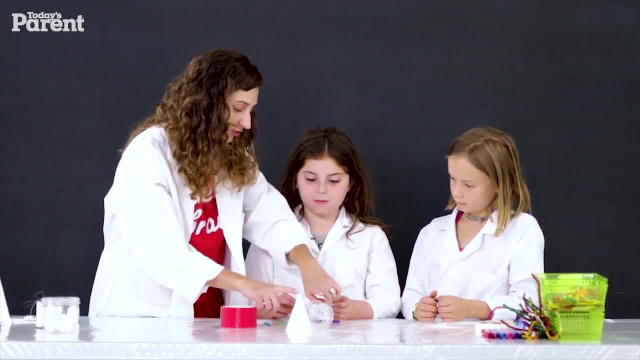 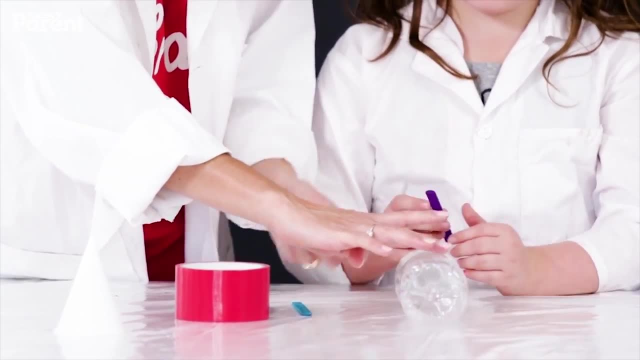 I'm going to get Mila to start first. Mila, will you put this stick just kind of along the water bottle somewhere here, And I need it to be sticking A little bit further than the top of there And I'm going to peel a piece of duct tape. 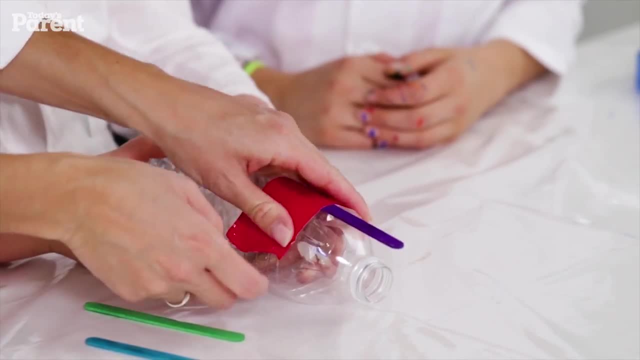 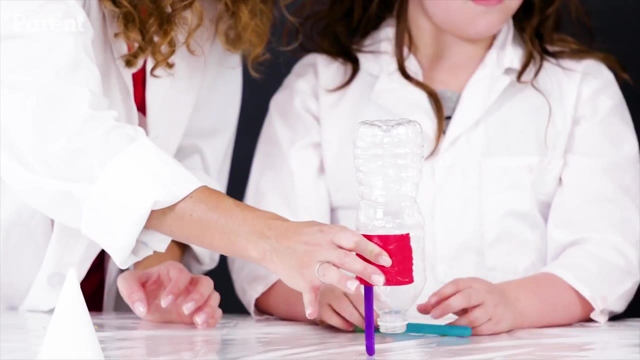 And then I won't get your fingers and I'll put that right there. Good job, We want it to be longer, because this is going to be the stand. Does it look like you can help hold it up? Do you think we need something else, though? 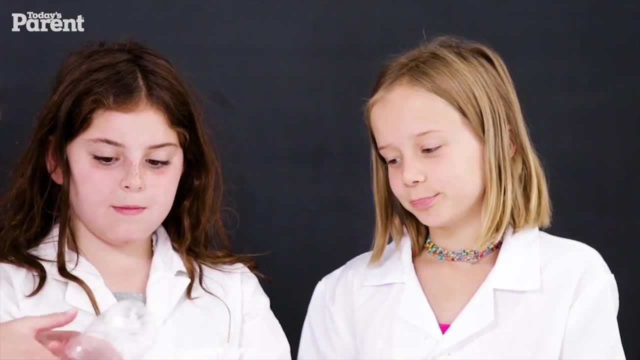 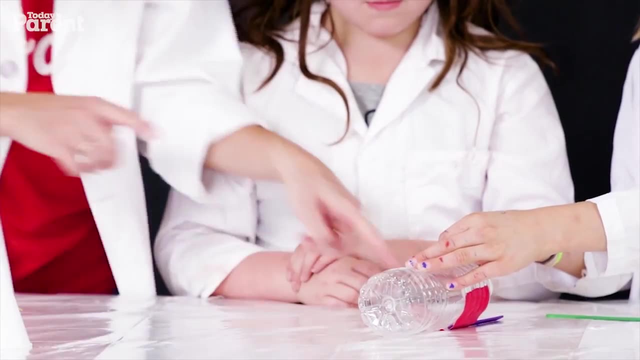 We need more Popsicle sticks, Exactly. Okay, it's your turn, Sophie. Do you want to find another spot, maybe right around there where my hand is, And we want to measure it up. so it's kind of the same. 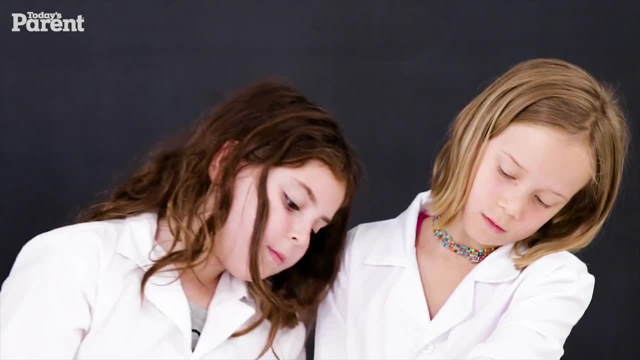 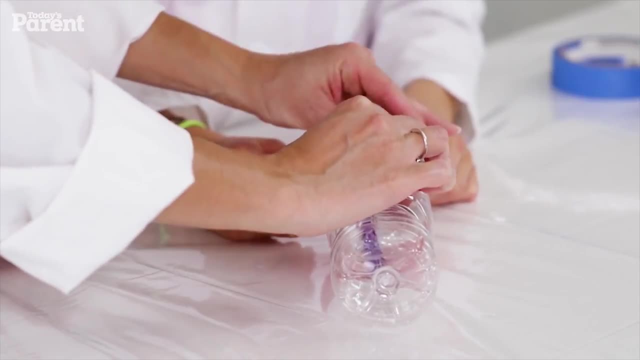 Like that. That looks great. Does that look? It's about the same distance as the purple one. Yeah, Yeah, Can I come in there? I think that's really good And we can always readjust it if we need to. 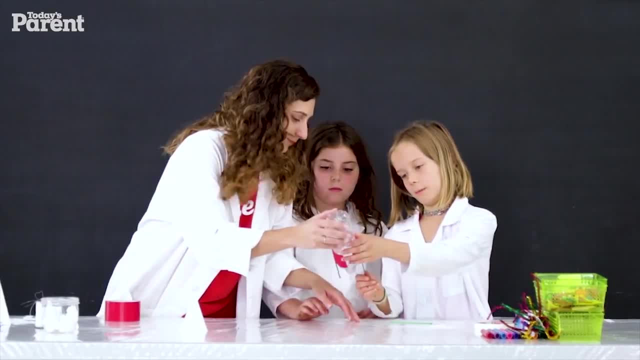 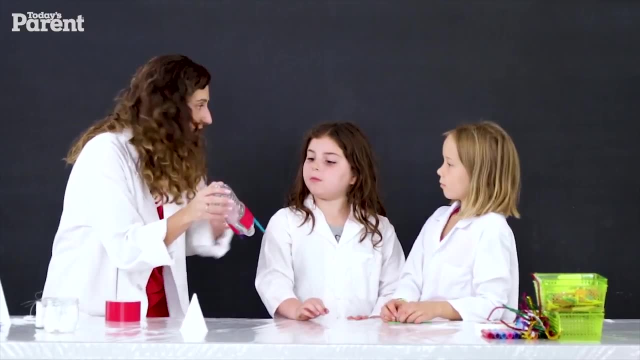 That's looking pretty good. What do you think? And let's do one more, Just a little bit bigger, A little bit. You know what I think it'll stand. Let's try with the third one, and if we feel like we need to adjust it, we'll just take the tape off. 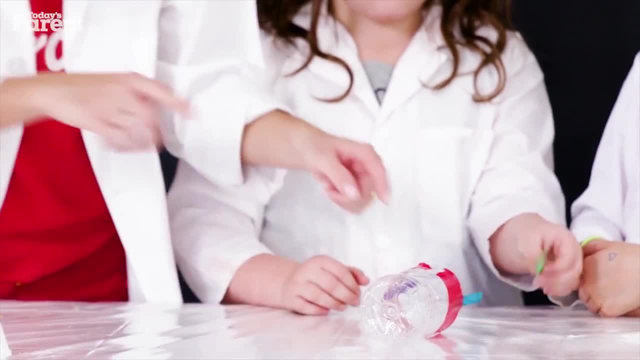 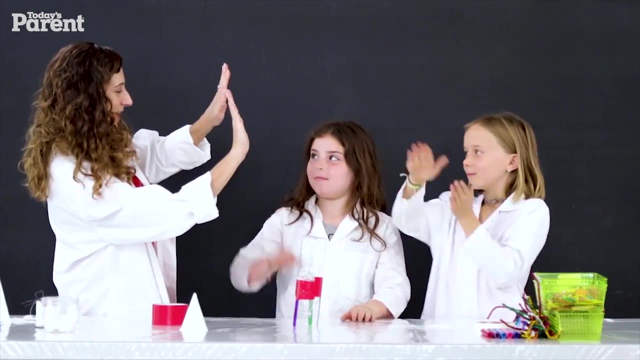 Okay. So, Mila, do you want to help with this? I think you can put this one right there and measure it. Yeah, Boop boop, boop boop. What do you think? Yay, Can I get a double high-five going over here? 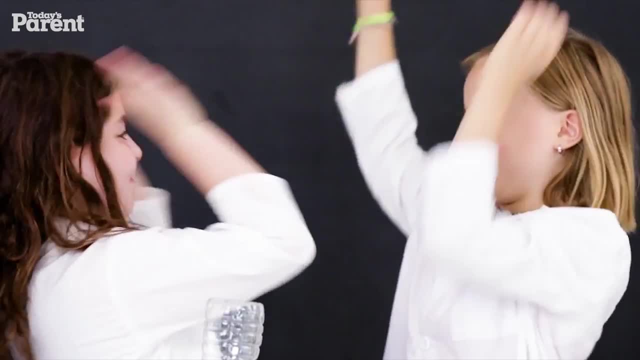 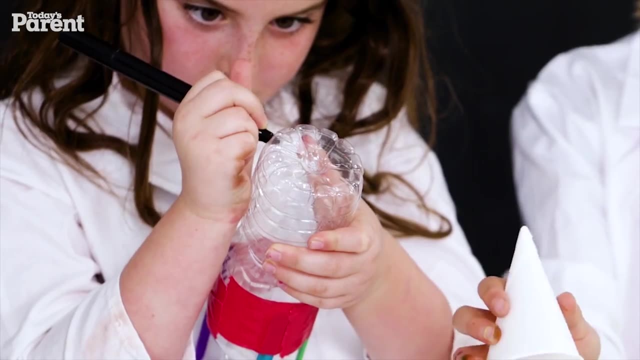 Yeah, And then you two give yourselves a high-five- Okay, awesome. And then we want to add this. To me it looks a little bit plain. Should we decorate this a little bit more? Yes, Can I draw on the bottle of faith? 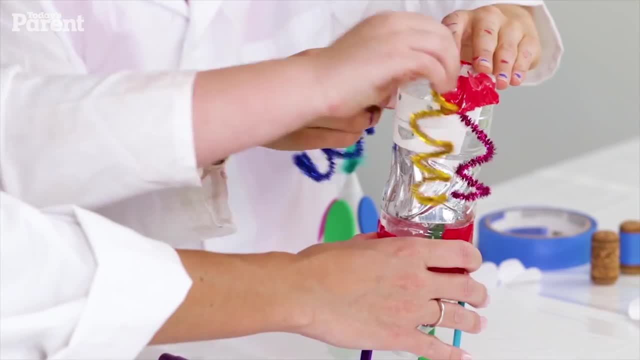 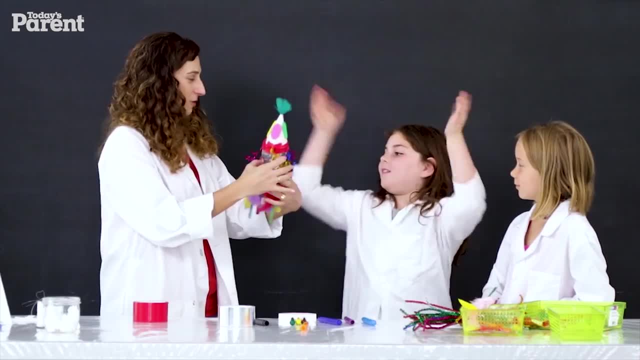 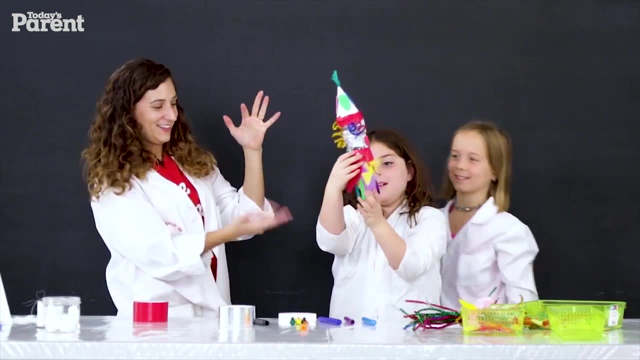 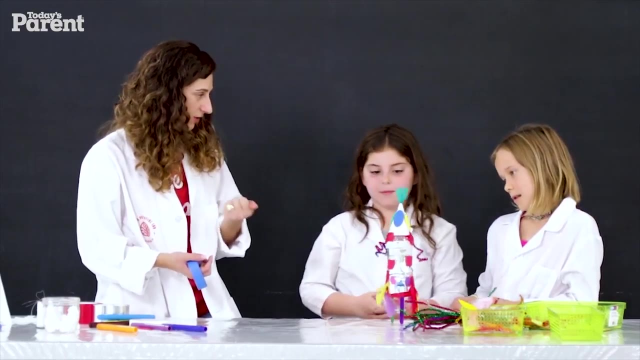 Do, do, do, do, do. This looks so good. Okay, do you want to present it? Ta-da, Okay, I have one last step. So do you notice? does this water bottle have a cap to it to close it? 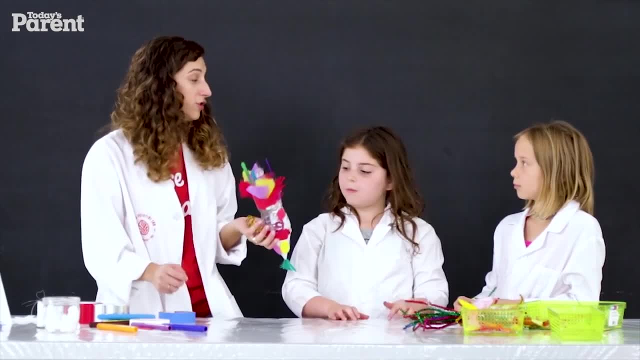 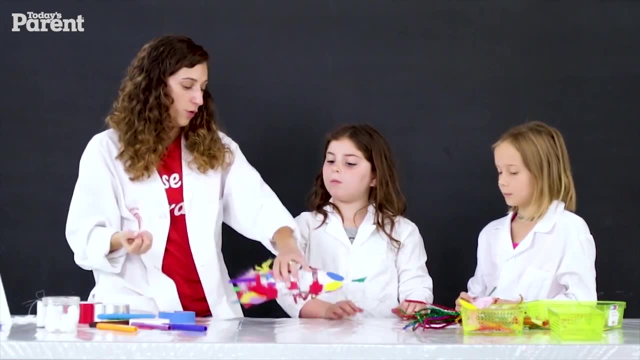 No, No, it doesn't right. That's because we're going to use this to put those baking soda pouches inside, But we do need something to close it tight tight. So what we have here is a cork, A cork.